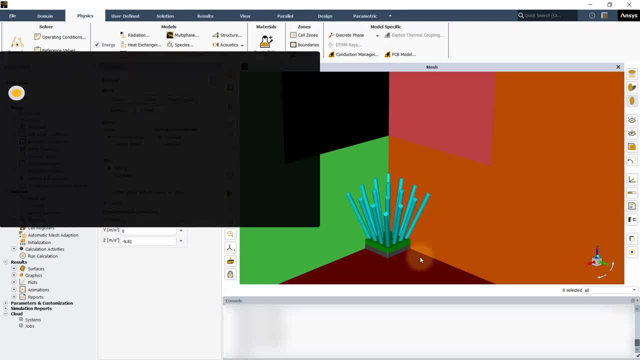 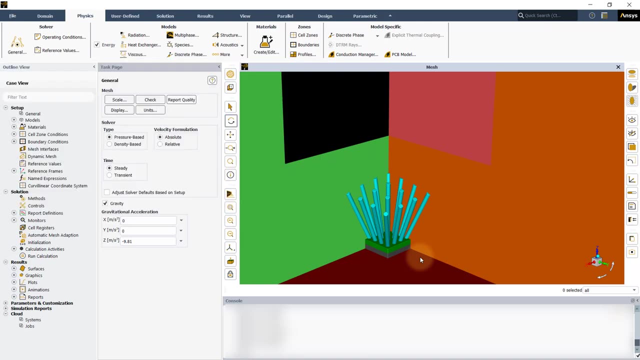 First, when you define boundary conditions, the value you enter is p prime, not p. And second, when you display contours or report pressures, you'll be getting values of p prime. So now that you know what happens when gravity is turned on, let's talk about density. 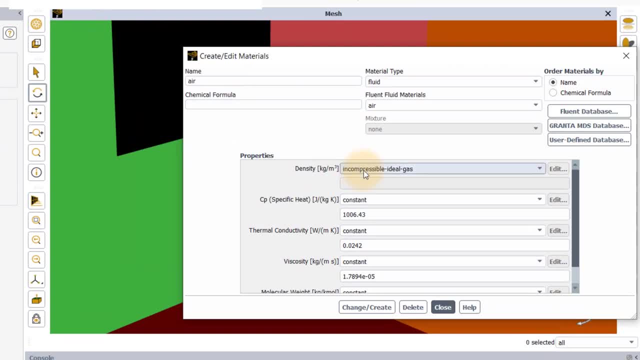 For natural convection. you can use any temperature-dependent density definition, including any of the real gas models, piecewise, linear and linear. However, the most commonly used models are Boussinesq, incompressible ideal gas and ideal gas. 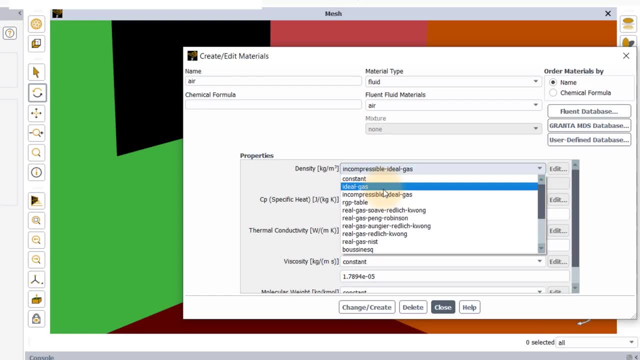 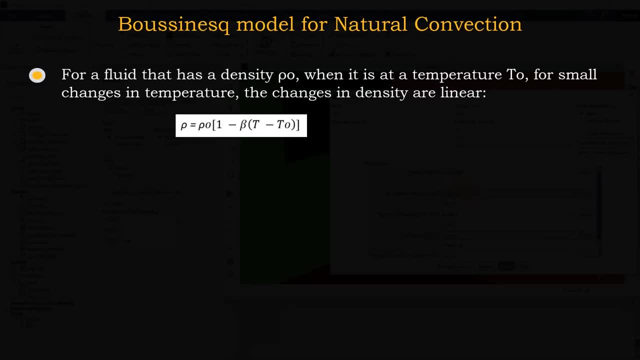 Both of the ideal gas models are discussed in another video, so I will only talk about the Boussinesq here. It is based on the idea that if the density of the fluid at a temperature T naught is given by row naught, 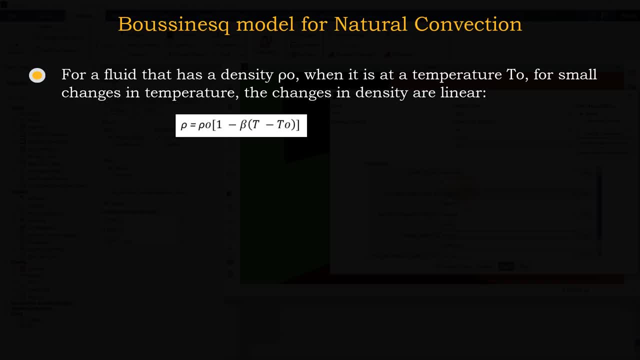 then, for small changes in temperature, the density of the fluid at a temperature T naught is given by row naught. Then, for small changes in temperature, the density of the fluid at a temperature T naught is given by row naught. The corresponding changes in density are linear and can be written like this: 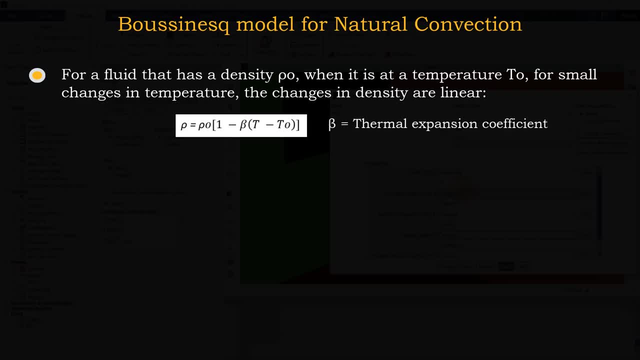 where beta is the thermal expansion coefficient. You can see that if we rearrange this and multiply by gravity, the left-hand side is the same as the body force term that we looked at before. so what happens in fluent is that it just replaces the body force term with the right-hand side of this equation. 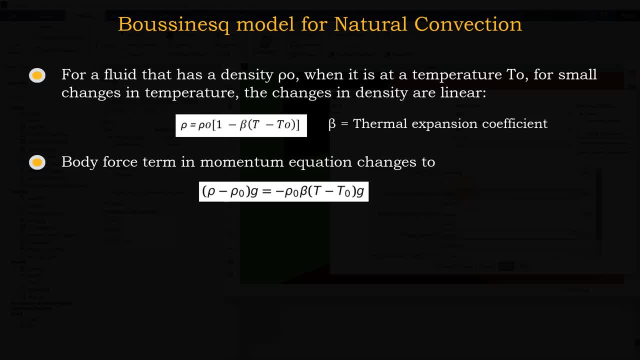 Linear variation of density is only realistic over a small temperature. Linear variation of density is only realistic over a small temperature. Linear variation of density is only realistic over a small temperature. so it's recommended to use the Boussinesq model when the product of beta and T-T naught is small. 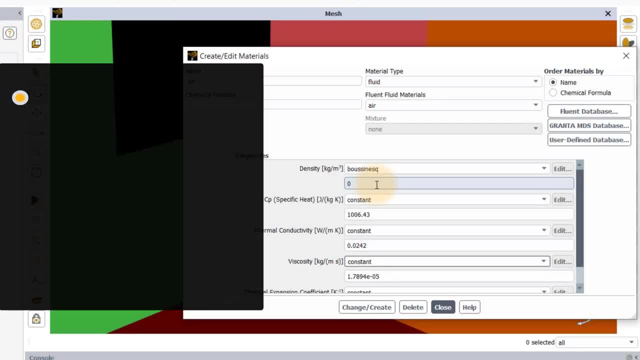 The advantage of the Boussinesq model is that it allows a constant density to be used, in the other terms, in the momentum equation, which can often lead to faster convergence. This might also seem like a lot of detail, but Boussinesq is one of the most frequently used models in natural convection. 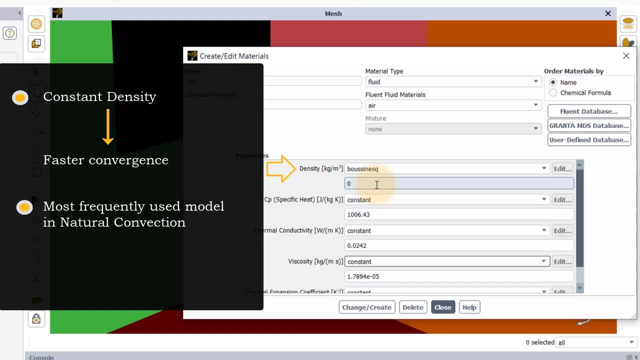 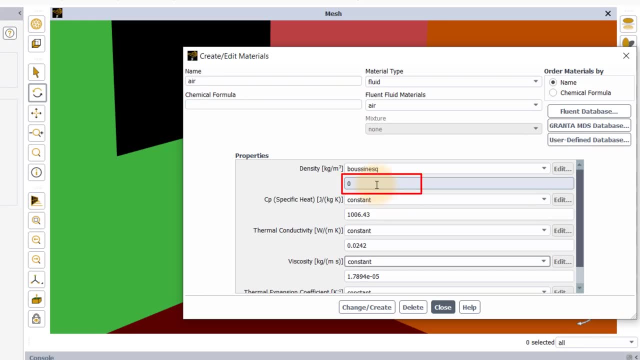 and it is important so that you'll know what to enter in the panel panel. First, when you choose Boussinesq in the materials panel, the value that you enter here is rho-naught in the equation that we were just looking at. The default value is zero.